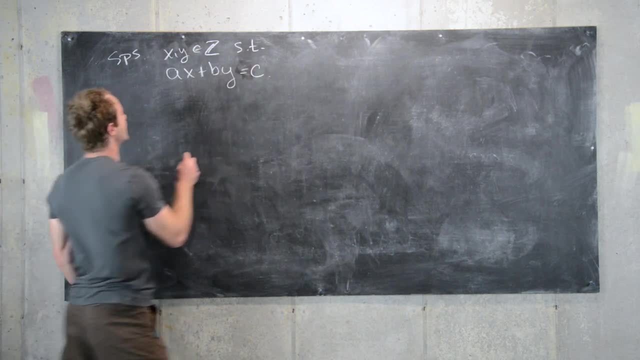 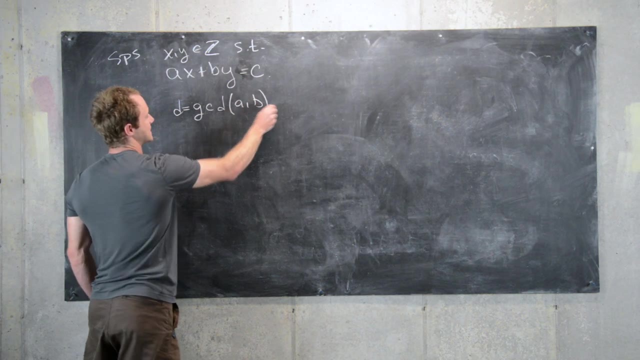 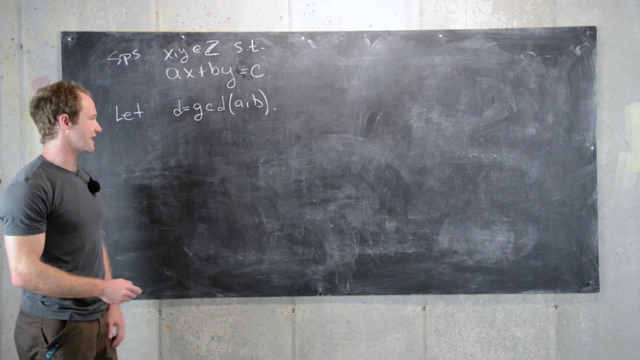 equation exists, Good. And then the next thing we want to do, let's say: let's let D equal the GCD of A and B. So, as we talked about before, we do have a solution if C is equal to D. but we want to consider a more general case here. Maybe C is not equal to. 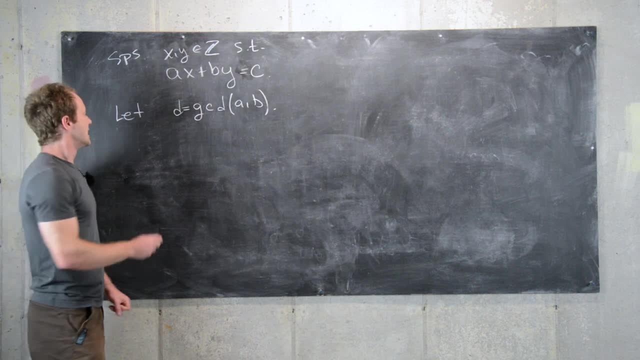 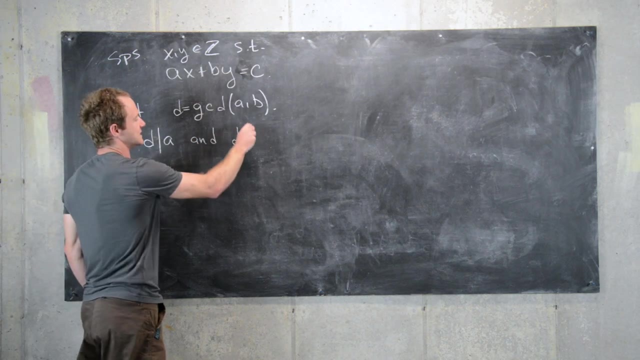 D, So we'll let D be the GCD of A and B. And so, notice, that tells us the following: That tells us that D divides A and D divides B, So it's the greatest common divisor, but it's also a common divisor. 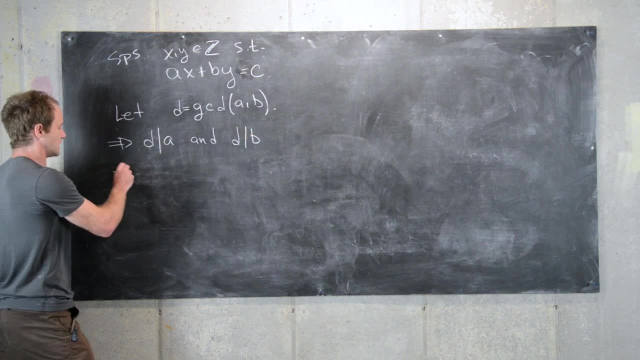 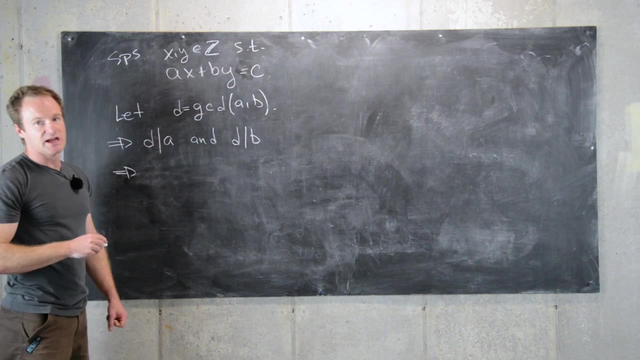 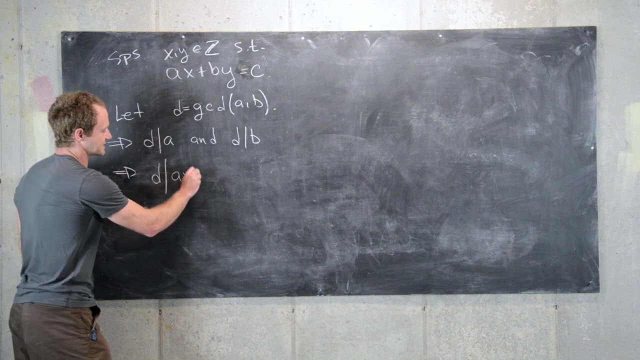 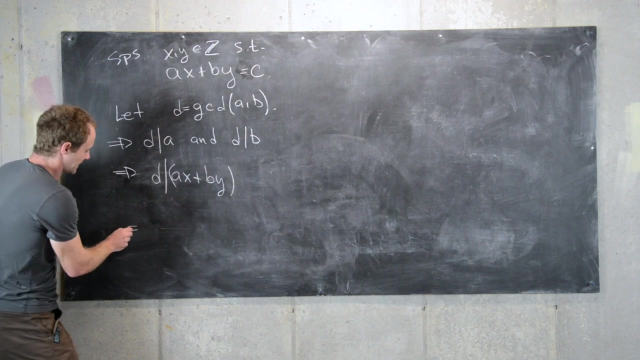 Good, So now that tells us that D divides any multiple of A and D divides any multiple of B, and thus it divides any combination of A and B. like this, so that we have: D divides AX plus BY, But that means that D divides the left-hand side of this equation, but that 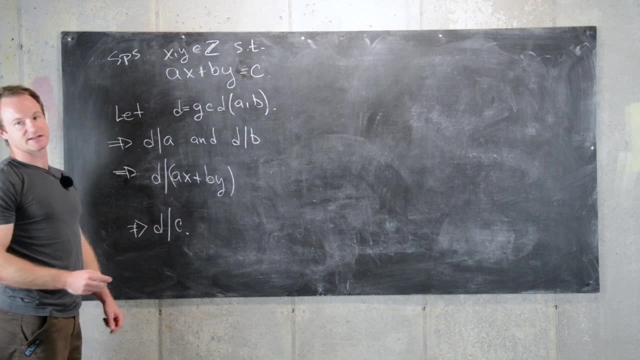 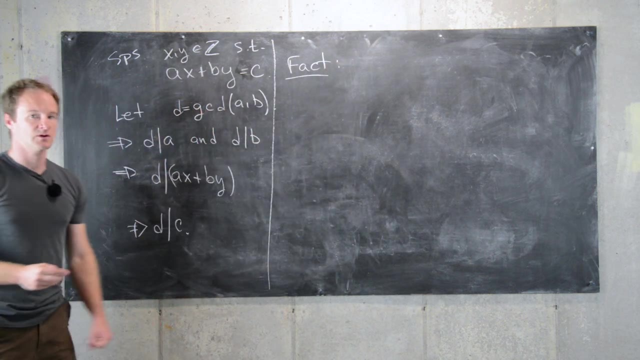 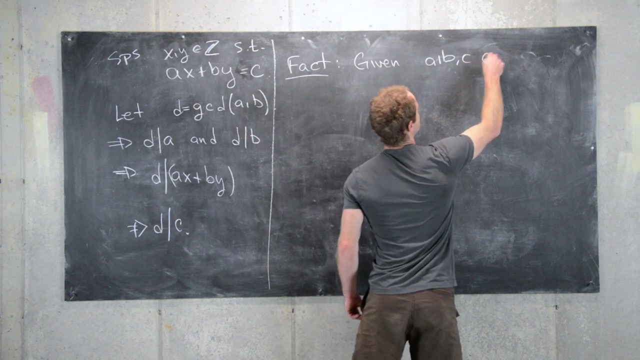 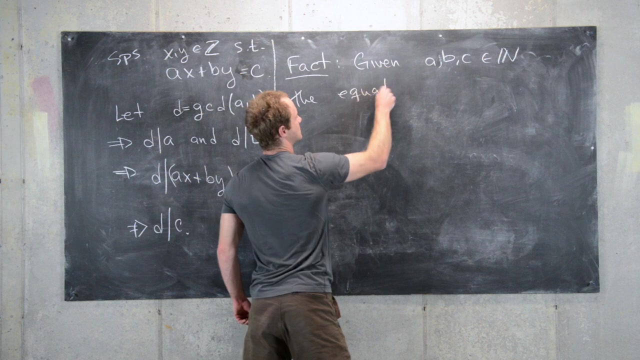 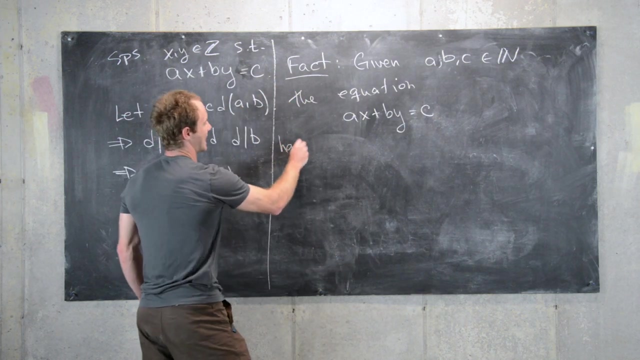 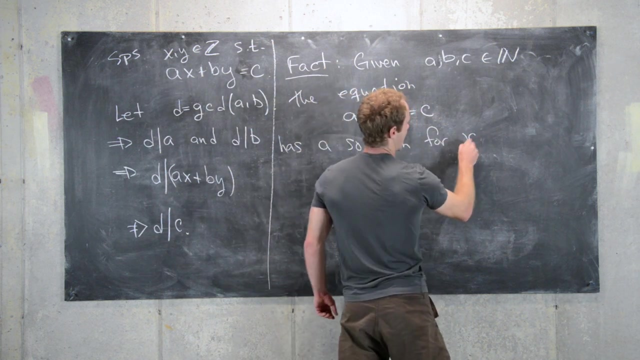 tells us that D must also divide the right-hand side of the equation. So that leads us to the following fact: which is given A, B and C natural numbers, the equation AX plus BY equals C has a solution OK For X. 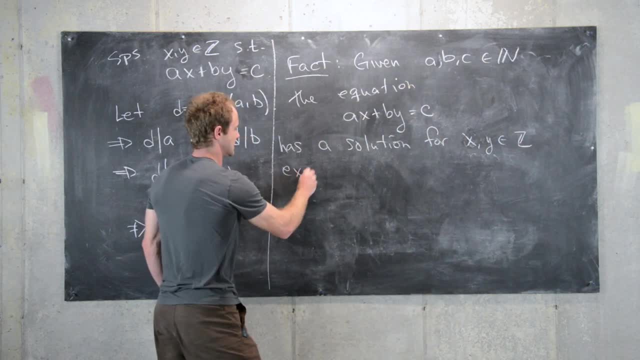 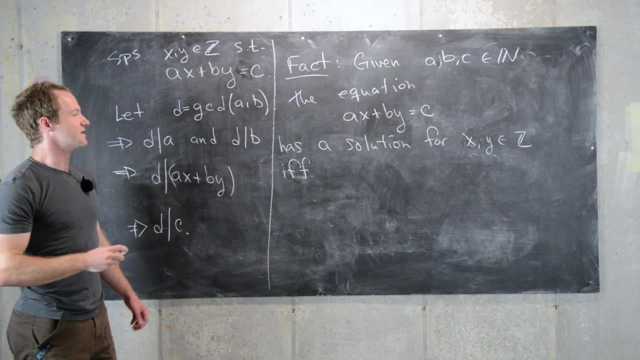 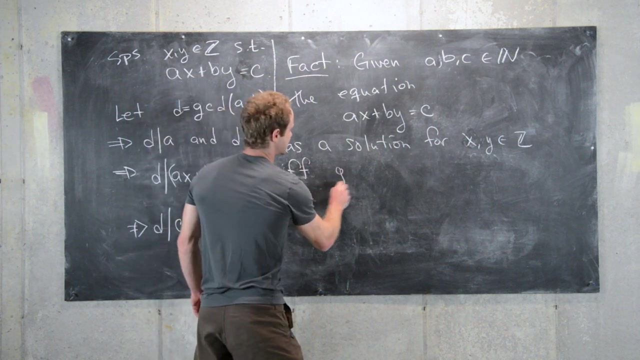 and Y in integers, if and then I'm going to put if, and only if, here, Although we haven't proven this super carefully, but we've given a lot of evidence to suggest this. If, and only if, the GCD of A and B divides C. 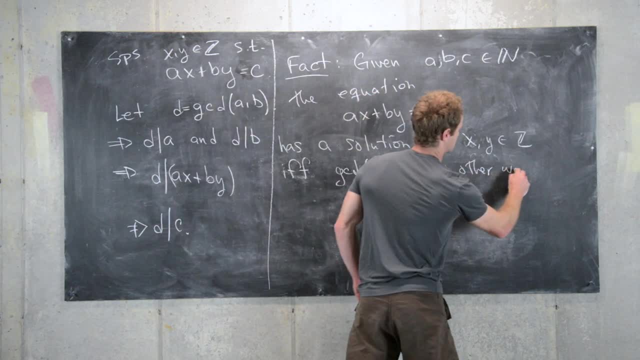 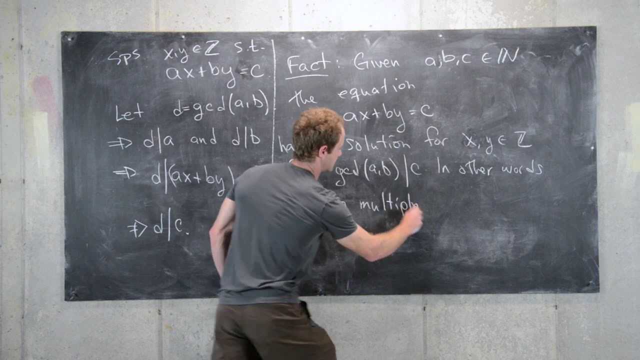 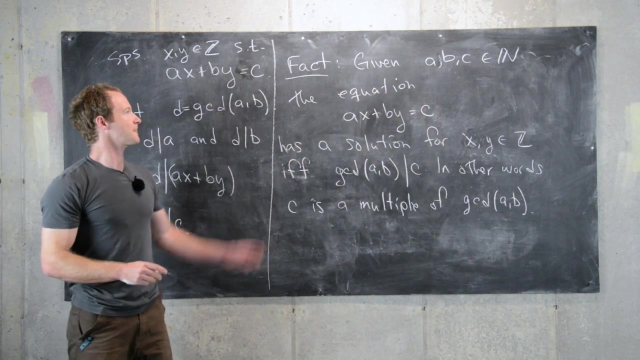 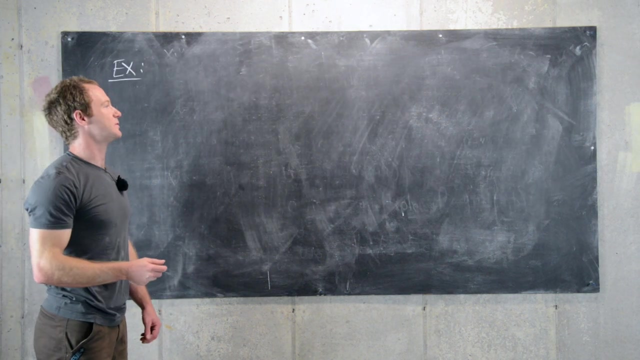 In other words, C is a multiple of the GCD of A and B. Okay, good So, now that we've established this fact, let's look at some examples. Okay, so let's look at some examples of linear Diophantine equations with solutions and without solutions. 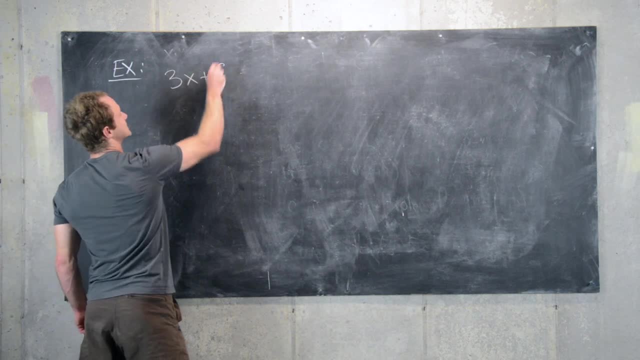 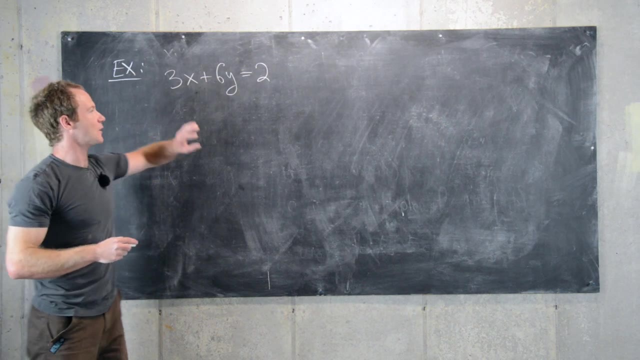 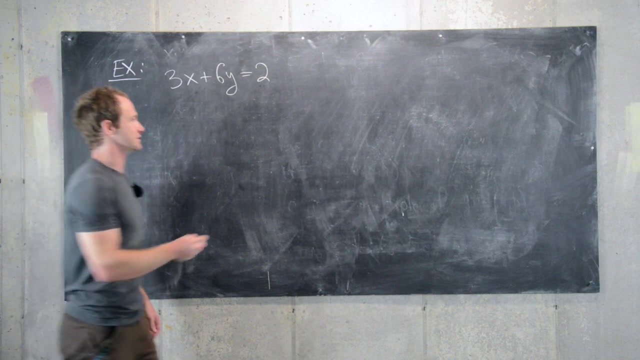 So let's first look at: 3x plus 6y equals 2.. So, recall, this has a solution if, and only if, 2 is a multiple of the GCD of 3 and 6, but it's not, so there is no solution. 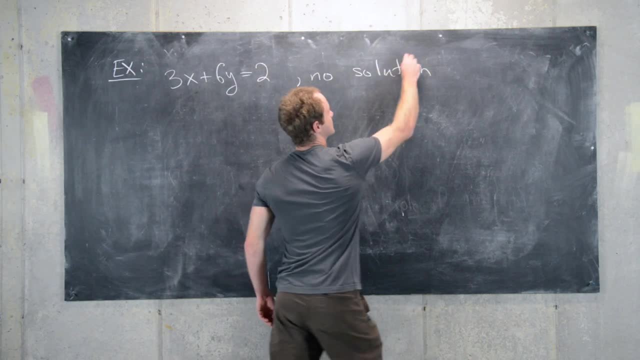 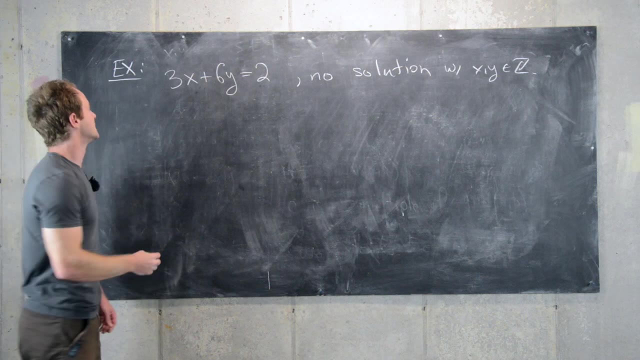 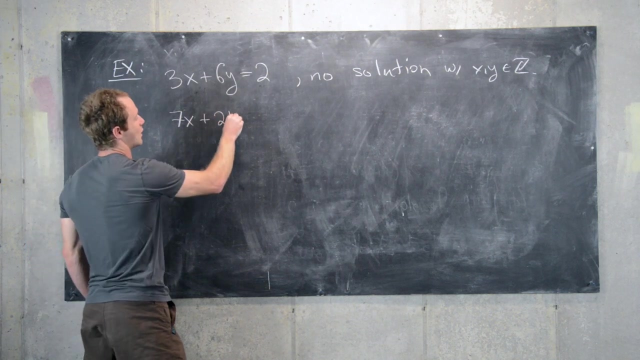 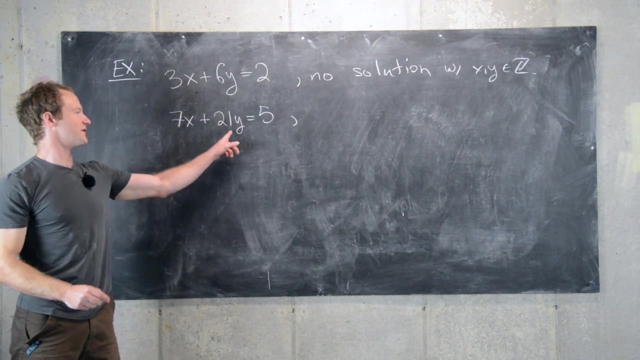 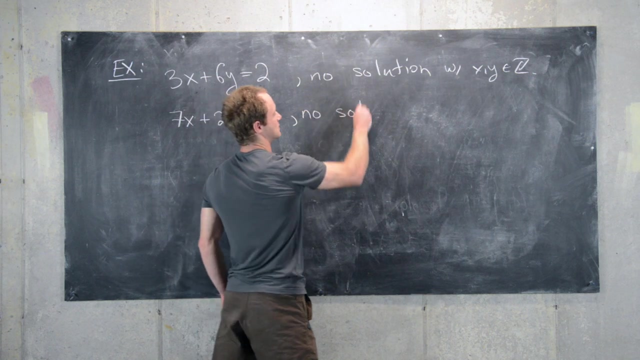 So no solution with x and y in integers. Good, So now Let's look at: maybe 7x plus 21y equals 5.. So again, since the GCD of 7 and 21 is 7, and 5 is not a multiple of 7,, there's also no solution with x and y integers. 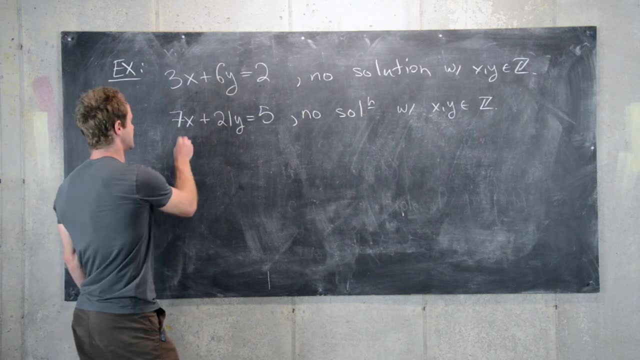 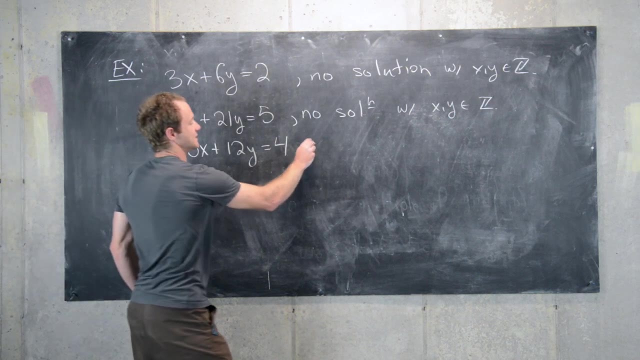 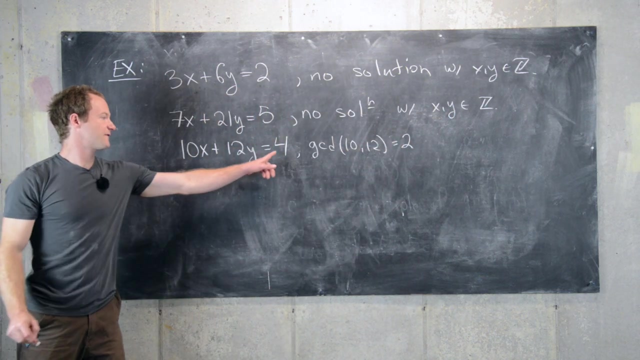 So let's look at one more example. So maybe 10x plus 12y equals 4.. So notice the GCD of 10 and 12 equals 2, and 4 is a multiple of 2, so we're guaranteed to have a solution. 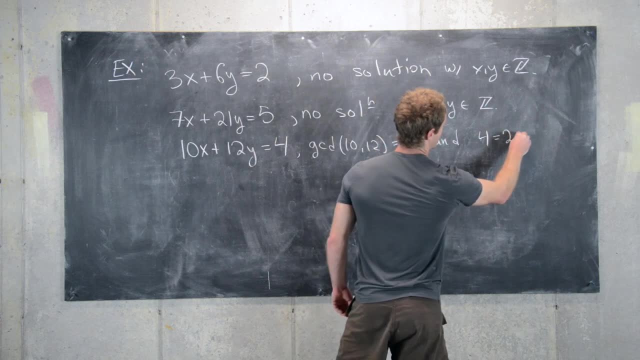 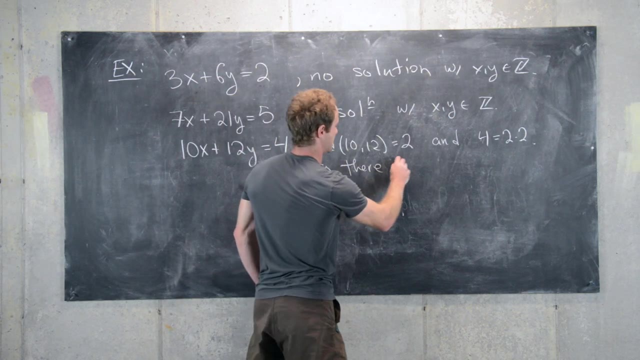 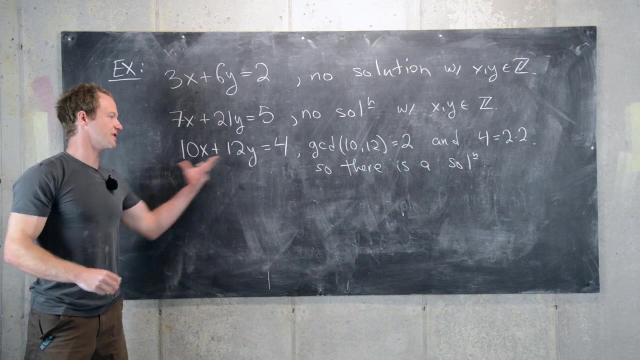 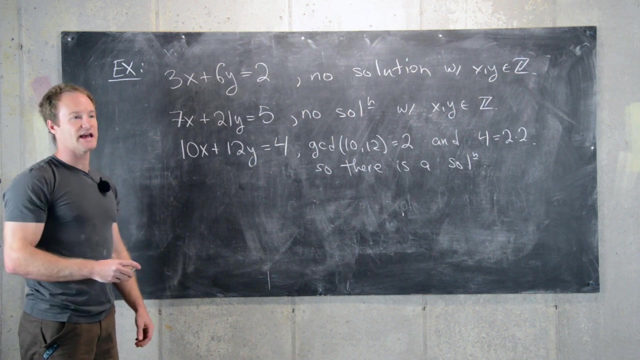 And 4 equals 2 times 2.. In other words, it's a multiple of 2, so we have a solution, So there Is a solution, So let's go ahead and find the solution. So now, obviously, we can do something like the extended Euclidean algorithm, but since these numbers are pretty small, we can guess a solution and check it. 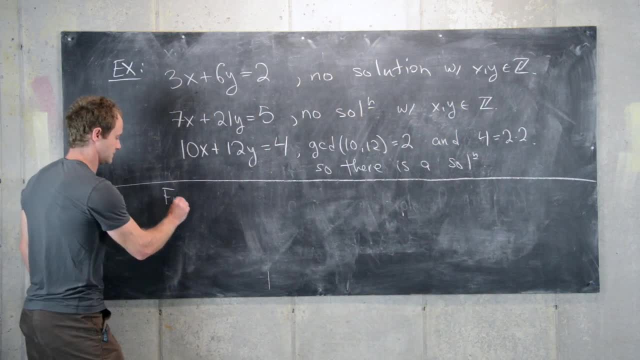 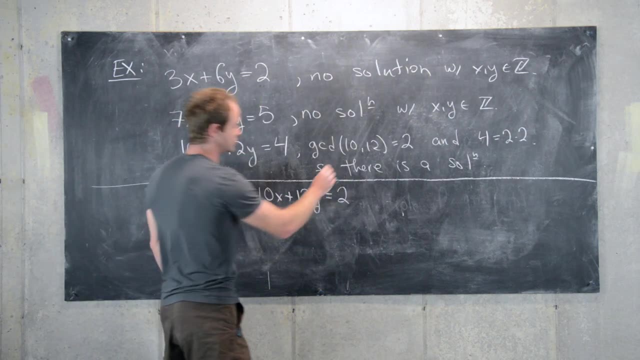 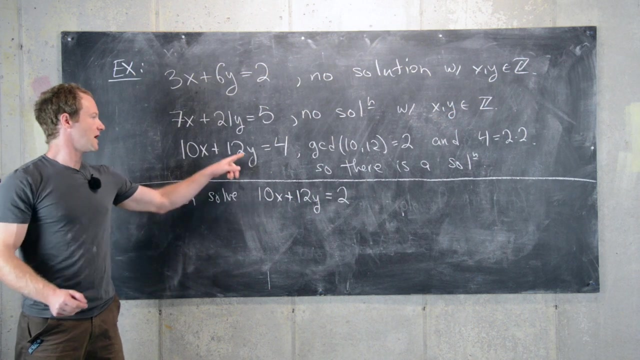 So maybe let's first solve: 10x plus 12y equals the GCD, Okay. And then notice: if we solve this equation, then we can multiply it by 2, and we've solved this equation, So this is pretty easy. 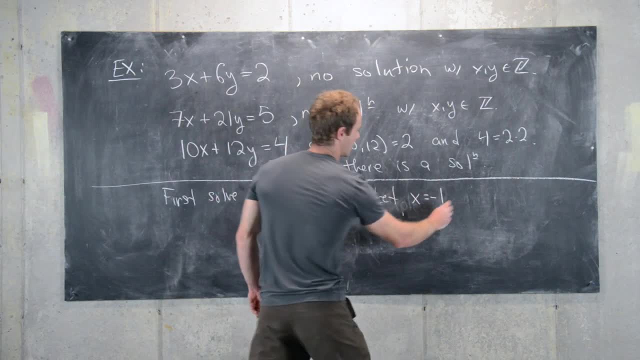 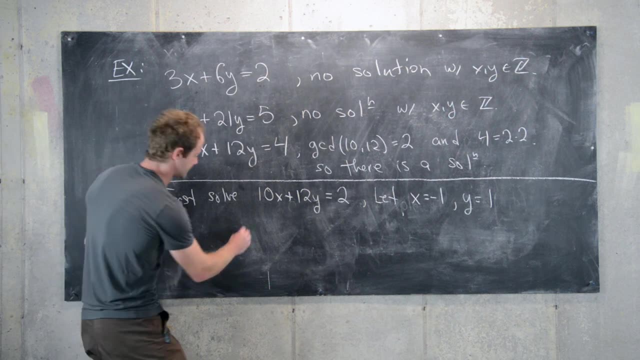 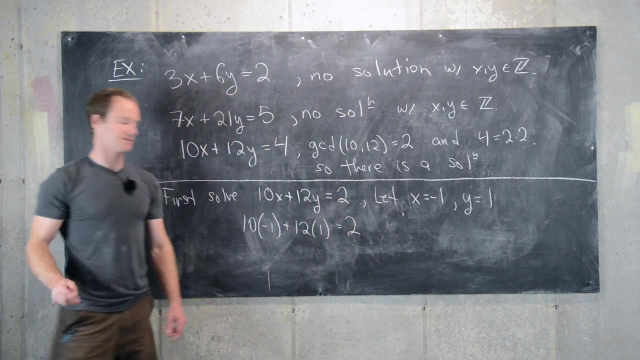 We can let x equal negative 1 and y equal 1.. Good, And that will give us a solution to this equation. So we'll have 10 times negative 1 plus 12 times 1 equals 2.. Good, Good. 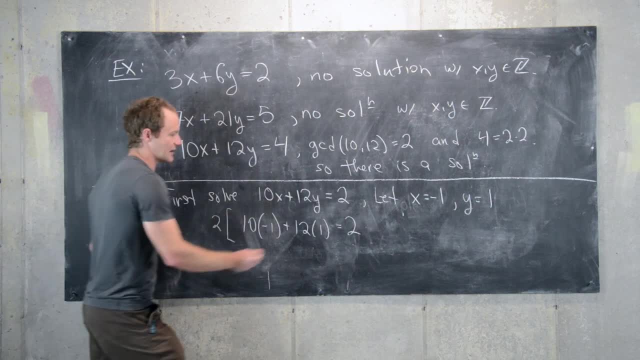 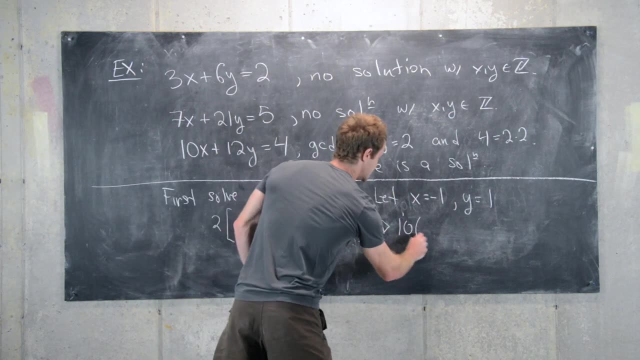 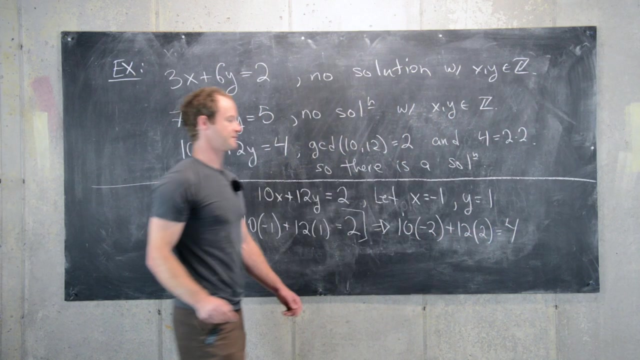 Now what we can do is Multiply this entire equation by 2, and then that's going to give us 10 times negative. 2 plus 12 times 2 equals 4.. And so we've solved the equation that we wanted to originally. 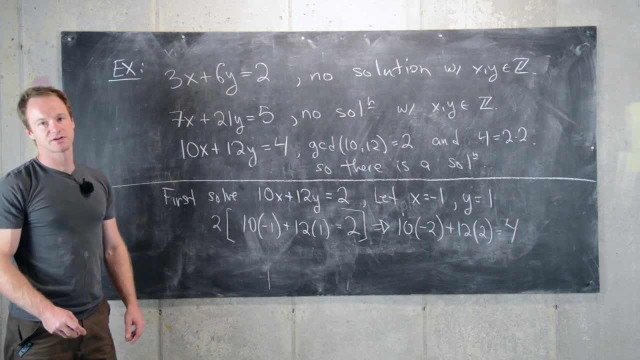 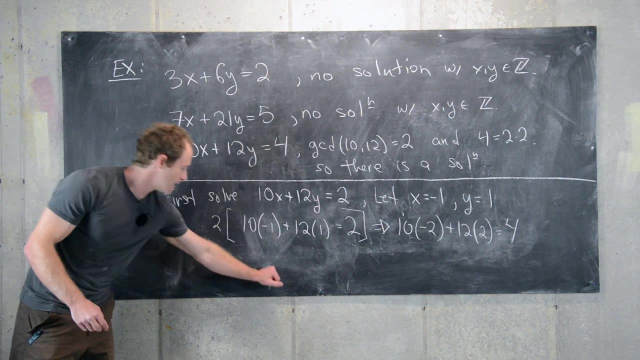 So now, next, let's see how we can get infinitely many solutions. So we'll notice that 10 and 12 have a least common multiple of 60. And then we'll write: 60 minus 60 equals 0.. 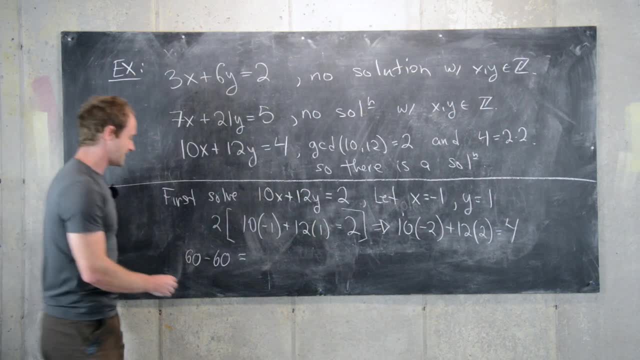 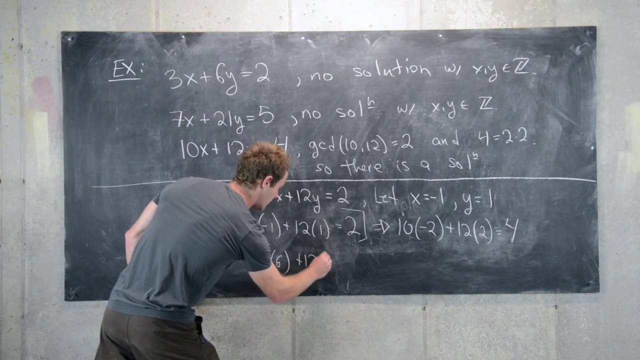 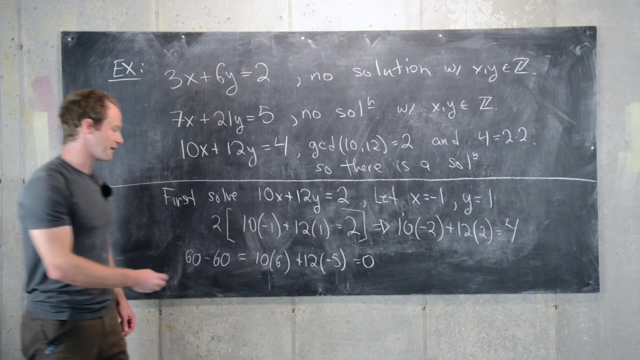 And then we'll factor 60 two ways. So let's factor 60 as 10 times 6 plus 12 times negative, 5 equals 0. And so since this equation is true, then we can also multiply it by k. 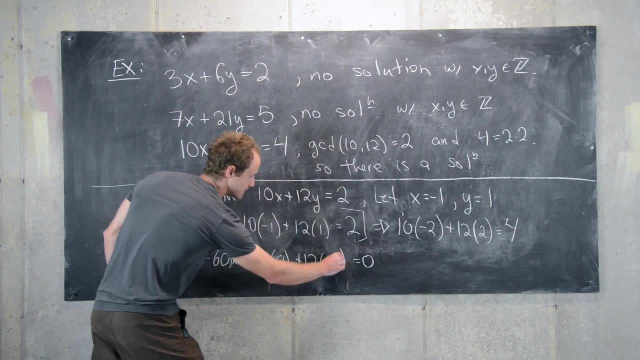 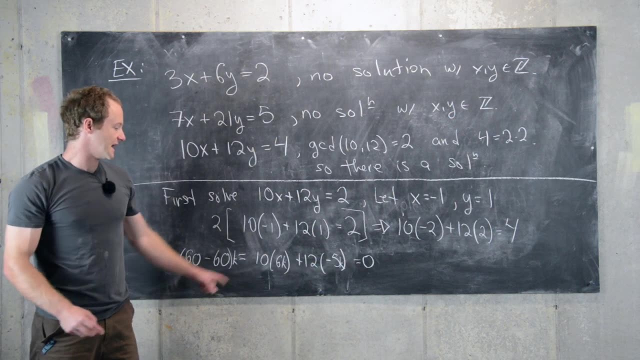 So 0 times k is 0. So we can multiply this by k, So we have 10 times 6k plus 12 times negative, 5k equals 0.. And now what we can do is we can take this equation and add it to our equation over here. 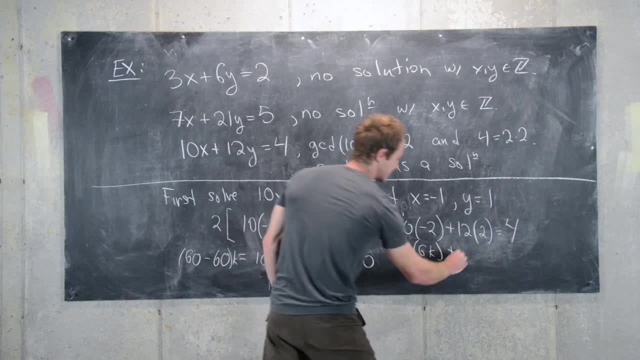 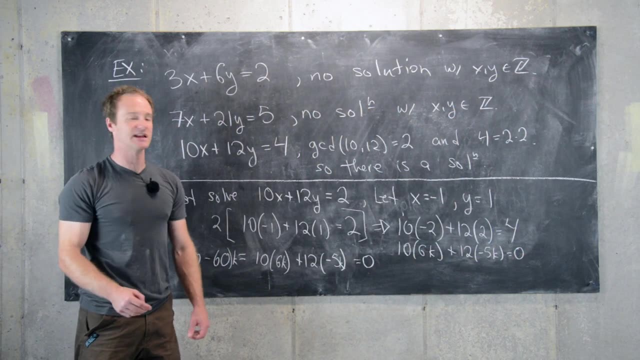 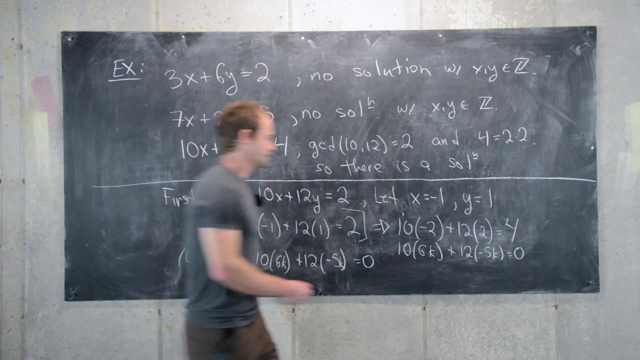 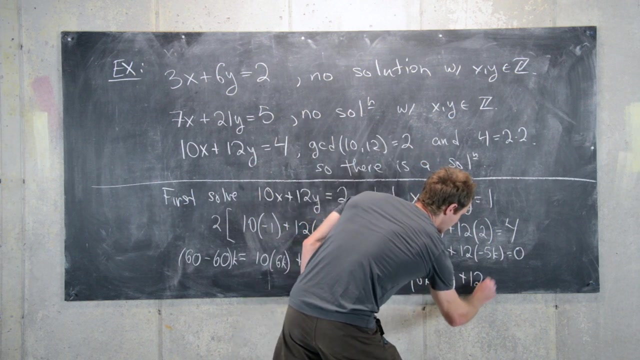 So we have 10 times 6k plus 12 times negative, 5k equals 0. And that's going to give us an equation that represents a family of all solutions To our original equation. So here we have 10 times 6k minus 2, plus 12 times negative, 5k plus 2 equals 4.. 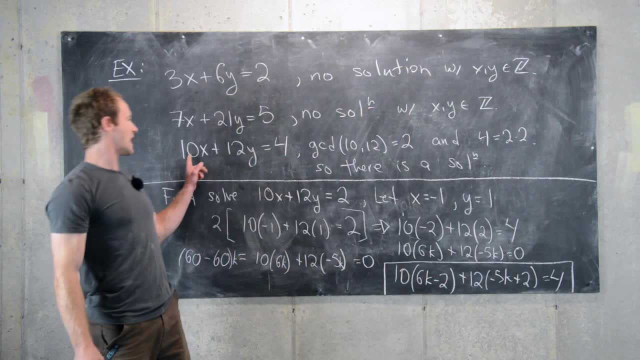 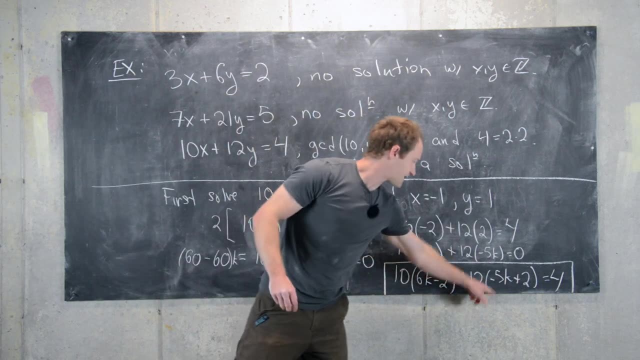 And now we have infinitely many solutions to our given equation. So we have: x is 6k minus 2.. Y is negative, 5k plus 2.. And k is any integer, Hence we would see 3.. So now we have different randomness equations. We can take these 500 out in our equation. This is as simple as she would show it to you. If you are been checking a video, What are you going to do? You know how to list numbers in your area. If you watched like this video, you will get the word Y. And you can change the number of numbers. Let me show you. So this n is 1 times 3 прав w. If you just close it and write, go back to where you started. That's the math.